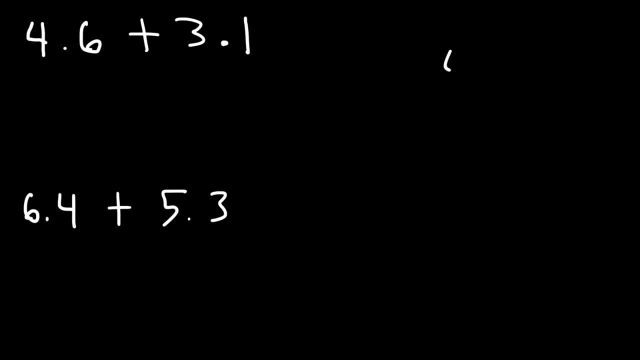 So let's start with this one. So let's set it up this way: 4.6 plus 3.1.. And starting with the first column on the right, we have 6 plus 1., Which is 7.. And then let's rewrite the decimal point, And now we can add 4 plus 3., Which is also 7.. 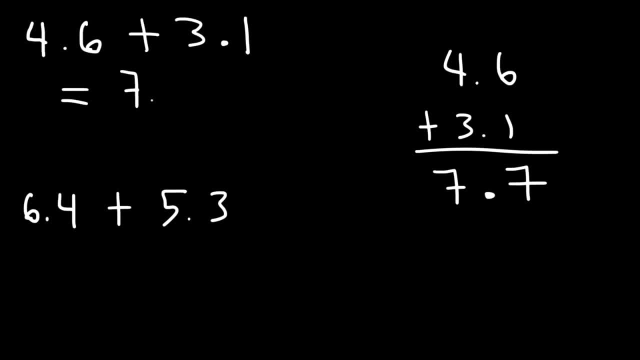 So the answer for the first example- 4.6 plus 3.1, is 7.7.. So now let's move on to the second example. So what is the sum of 6.4 plus 5.3?? 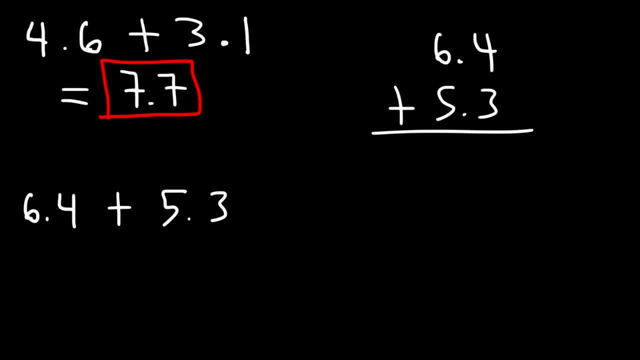 Well, we know that 4 plus 3 is 7.. And then we need to add 6 plus 5, which is 11.. So the answer for the second example is 11.7.. Now let's add decimal numbers that end in the hundreds place. 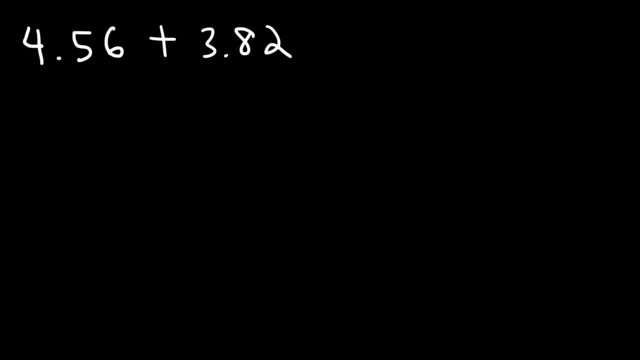 So let's try this example: 4.56 plus 3.82.. Feel free to pause the video and work on that problem. So first let's stack them together And then let's add 6 plus 2, which is 8.. 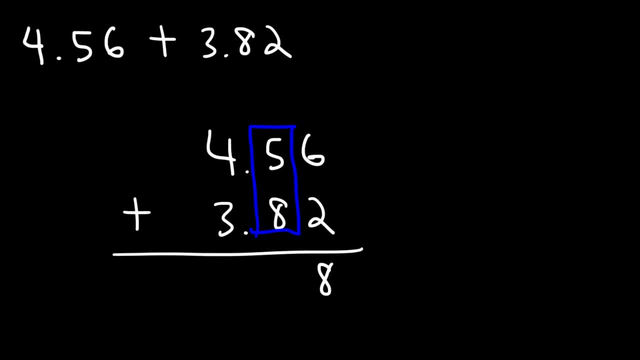 And then we have 5 plus 8.. That's 13.. Now what we need to do here is we need to write the 3 and then carry over the 1.. So in the last column we have 1 plus 4, which is 5. And 5 plus 3 is 8.. 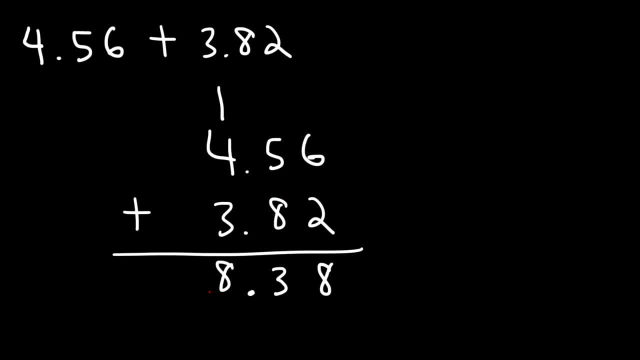 So the 5 plus 3 is 8.. And then we need to write the 3. And then carry over the 1.. final answer is 8.38.. And so adding decimal numbers is not too difficult, but let's try. 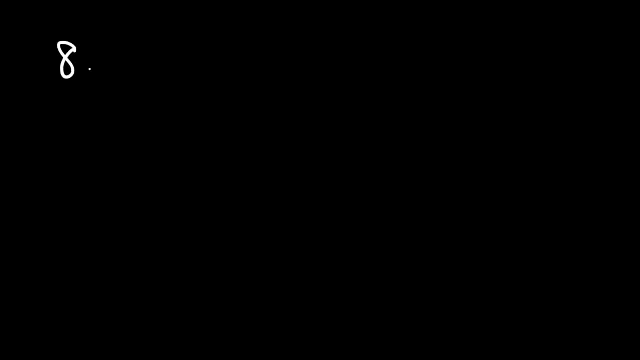 another similar example to this problem. So let's say we have 8.47 plus 7.96.. Feel free to pause the video and work on that example. So let's begin by lining up the two numbers And, as always, let's start with the column on the right side. So we have 7 plus 6, which is 13.. So let's write. 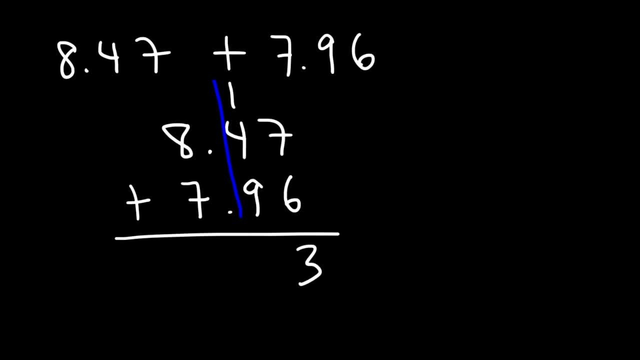 the 3, carry over the 1.. And then 1 plus 4 is 5.. 5 plus 9 is 14.. So we're going to write the 4, carry over the 1 to the next column, And then 1 plus 8 is 9.. 9 plus 7 is 16.. So the answer is: 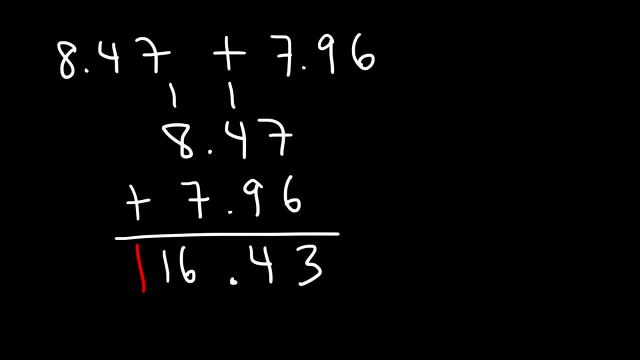 16.. 14.43.. And so that's it for this problem. Now let's move on to another example. So what would you do in a situation like this? Let's say, if you're given 7.34 plus 5.9.. So here we have a. 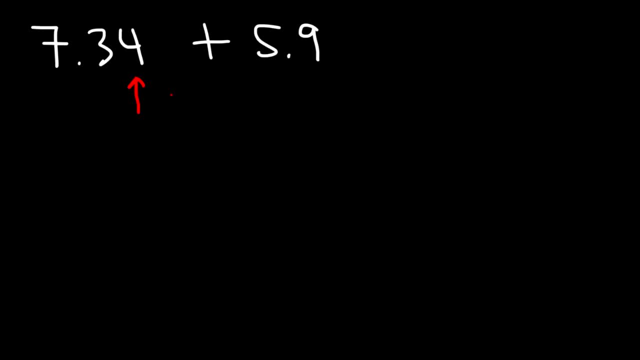 number that ends in the hundreds place and this one ends in the tenths place. So what would you do in this case? Well, when you write the two numbers together, make sure that the decimal points line up. So we need to stack them. 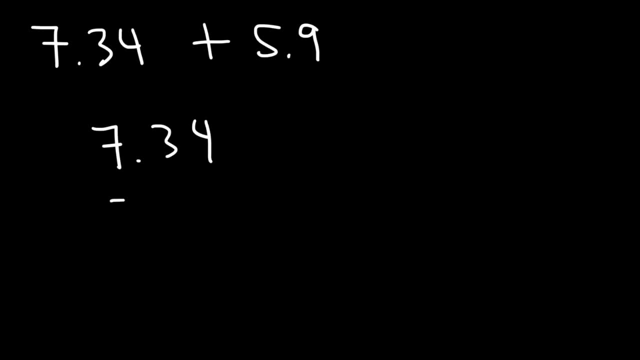 like this: Here it's 7.34 and the next one is 5.9.. So, as you can see, the decimal points are lined up. Now we don't have a number here, so we can put a 0.. 5.9 is the same as 5.90.. So let's add. 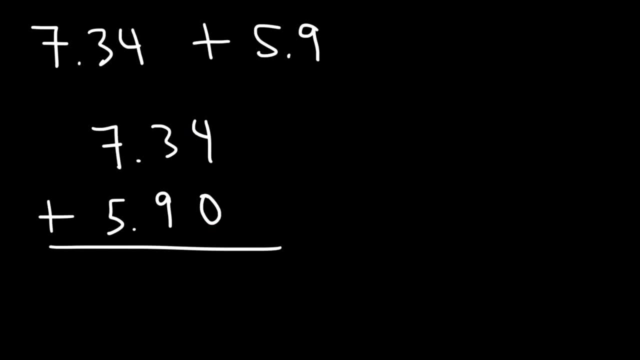 the first column, 4 plus 0 is 4.. And then for the second column, 3 plus 9,, that's 12.. And now we need to carry over the 1.. 1 plus 7 is 8.. 8 plus 5, that's 13.. So the 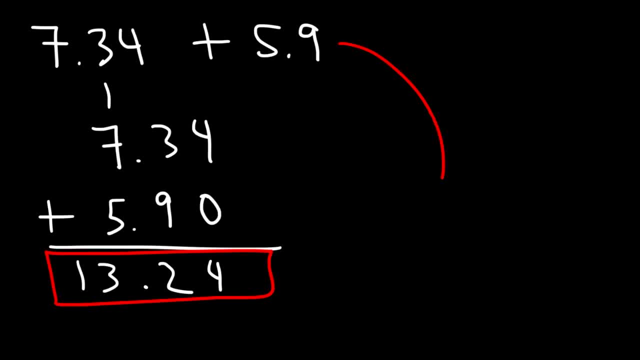 answer is 13.24.. Now for the next one. let's go ahead and add 14.7 plus 3.685.. So feel free to take a minute, pause the video and try that example problem. So let's go ahead and add up the two numbers, but we need to line it up. 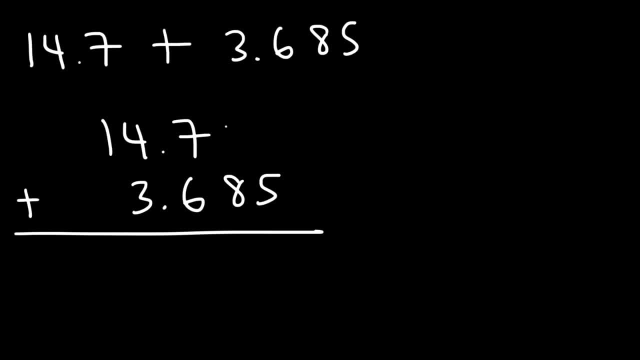 properly. So if you want to, you can add two zeros here, And so in the first column we have 0 plus 5, which is 5, and then we have 0 plus 8, which is just 8.. For the third column we have 7. 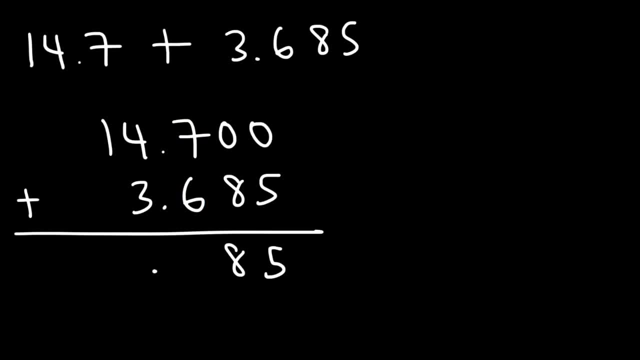 plus 6, so that's 13.. So let's write the 3 and then carry over the 1 to the column in the left, And then 1 plus 4 plus 3, that's going to be 8.. And for the last, 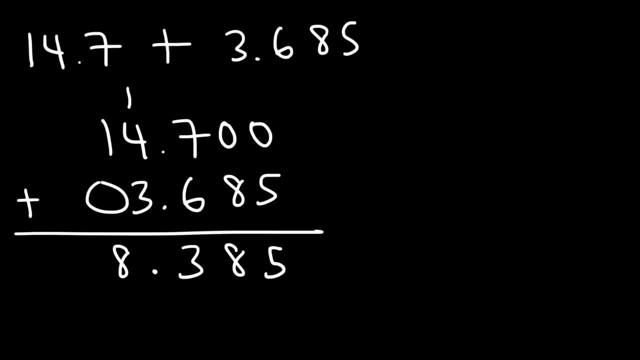 one, we could just bring it down. Or if you write a 0 here, 1 plus 0 is 1.. So the final answer is 18.385.. Now let's move on to the next example. So let's add 3. 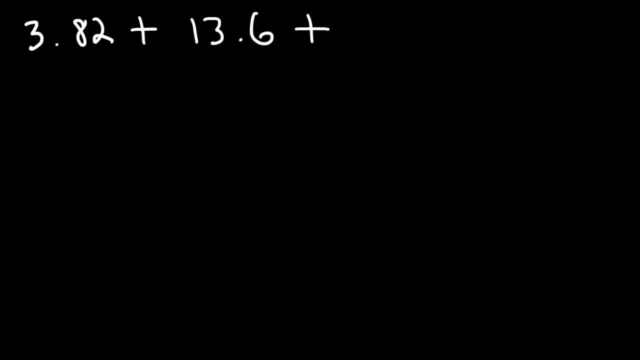 numbers, this time 3.82 plus 13.6 and 5.431.. So go ahead and work on that example. So let's begin by lining up the 3 numbers. So the important thing to keep in mind is to make sure that the decimal points are lined up. If you focus, 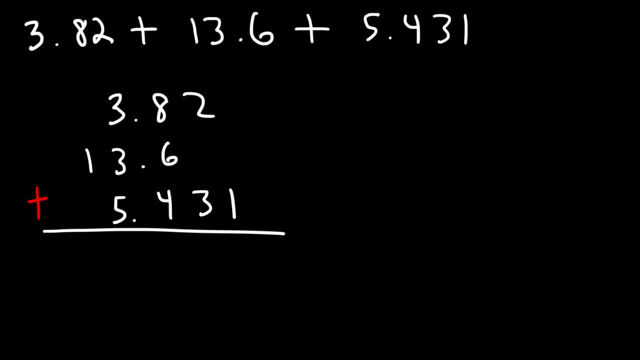 on that. everything else will be fine. Now let's add some 0s. So I'm going to add 1 0 here and 2 0s, just to make sure everything is aligned. Everything looks nice Now. in the first column we have 0 plus 0 plus 1.. And so 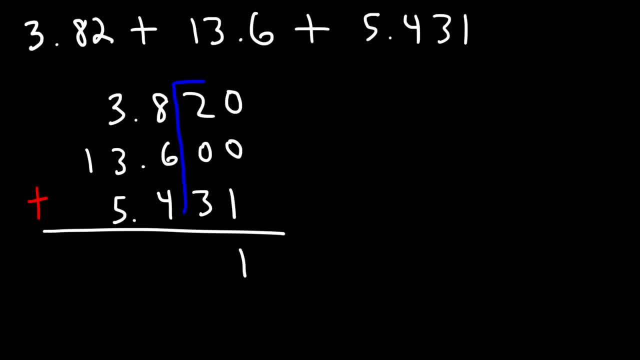 that's going to be 1.. And then for the second column, it's just 2 plus 3, which will give us 5.. Now, if we move on to the third column, 6 plus 4 is 10.. 10 plus 8. 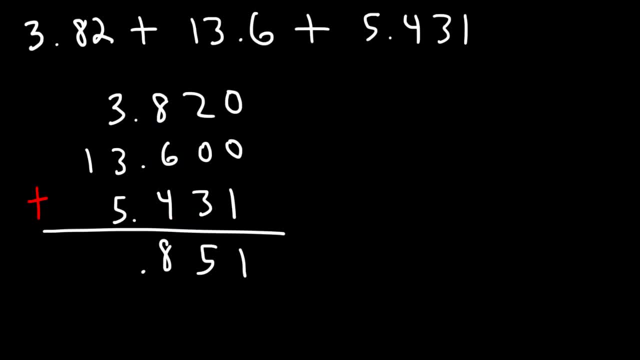 is 18.. So we're going to write the 8, carry over the 1.. Now we have 1 plus 3,, which is 4.. And then 4 plus 3 is 18.. So we're going to write the 8, carry over the. 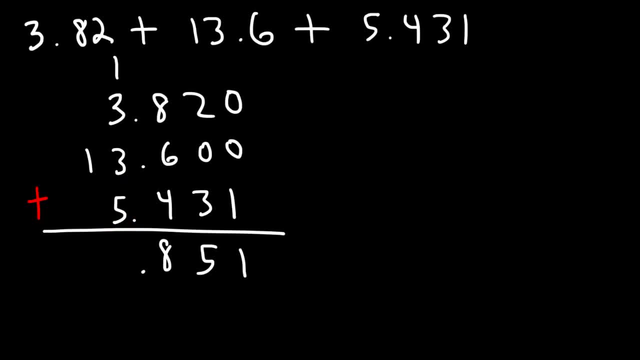 7. And then 7 plus 5, that's going to give us 12.. So let's write 2, carry over the 1.. 1 plus 1 is 2.. And so the final answer for this example is 22.851.. 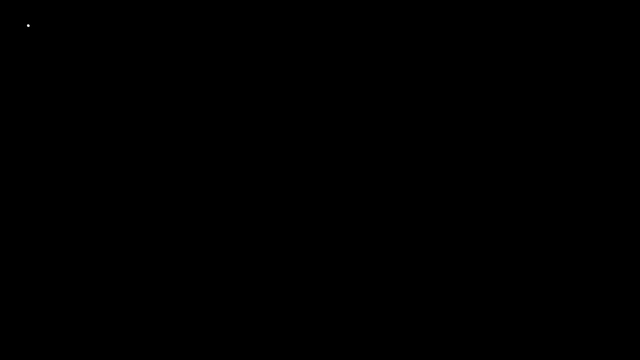 So here is another example: 7.643 plus 12.31 plus 126.3.. So for the sake of practice, go ahead and try that. So let's line up the numbers carefully. So the second one is 12.31.. And then the last. 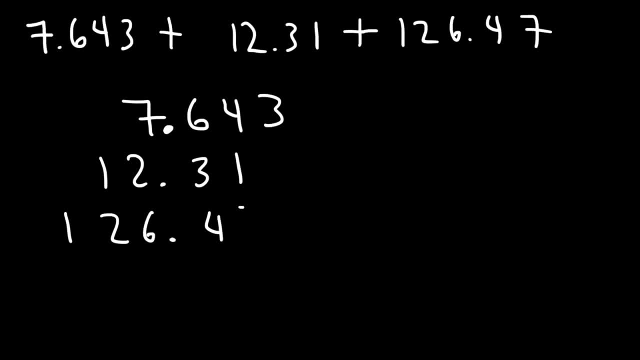 one is 126.47. And let's add 2: 0s. So in the first column all we have is a 3. And then for the second column we have 12.31.. And then the last one is 126.47.. And then 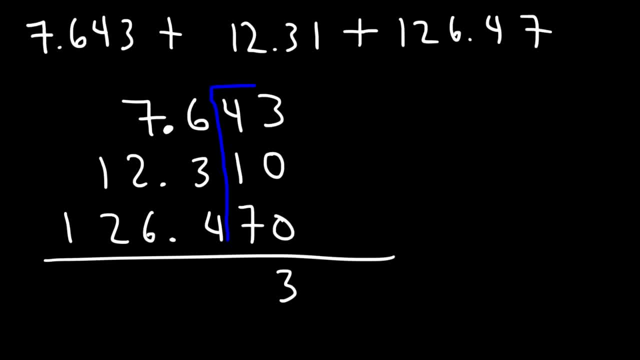 for the second column, all we have is a 3.. And then for the second column, all we have is a 3.. And then for the second column, all we have is a 4.. And then for the second column, all we have is a 3.. And then 4 plus 1,, which is 5.. And then 5 plus 7,, that's 12.. So let's. 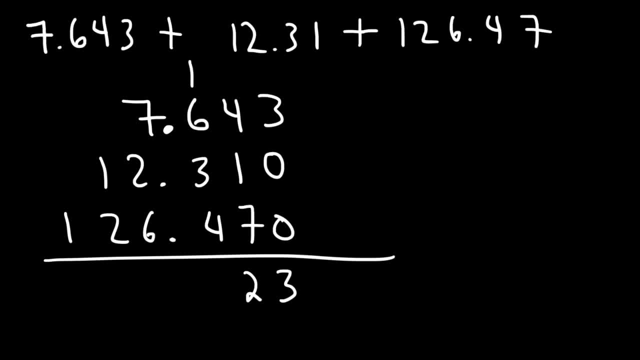 carry over the 1 and write the 2 at the bottom. And for the third column we have 1 plus 6, which is 7.. 7 plus 3 is 10.. 10 plus 4 is 14.. So let's write the 4 and put the 1 in. 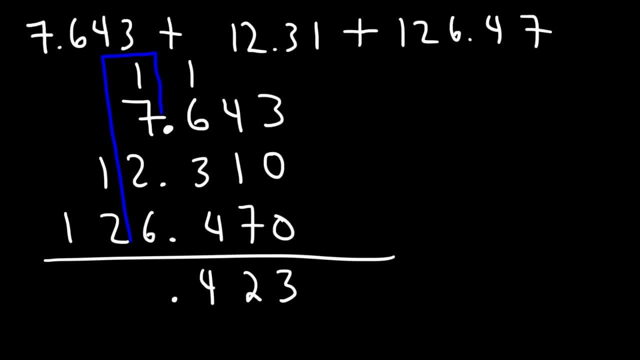 the next column on the left. And now for this column, we have 1 plus 7, which is 8.. And 8 plus 2 is 10 plus 6, so that's 16.. Let's carry over the 1, and then 1 plus 1 plus 2 is 4, and then 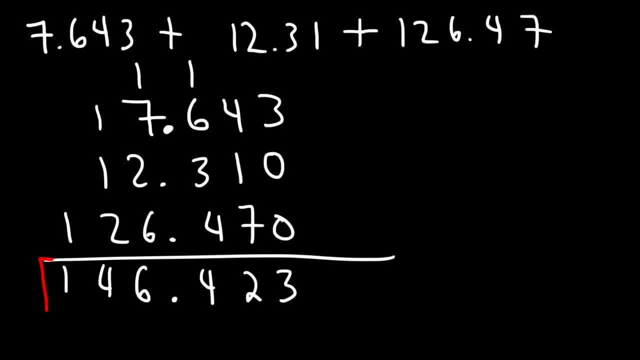 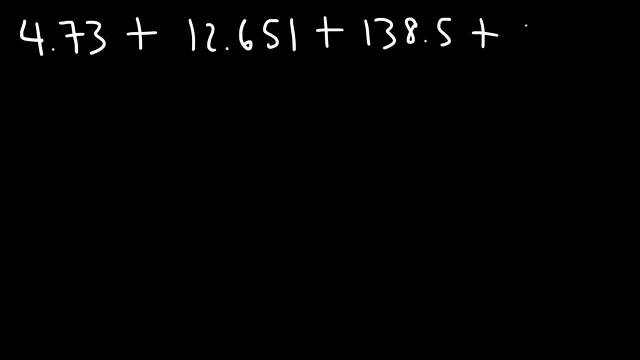 we can bring down the other one. So the answer for this one is 146.423.. So for the last example I'm going to make it a little harder than the other ones, because it's the last example, and so let's add 4.73 plus 12.651 plus 138.5 plus 0.9368.. So go ahead and give that problem a shot. 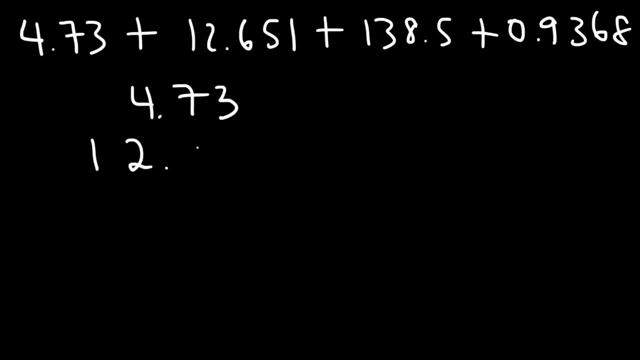 So let's begin by lining up the numbers, and then the last one is 0.. 0.9368.. So what I'd like to do, as you know, at this point is to fill in the other numbers with zeros to the right. So for the first column, all we have is an 8, and for the second column, 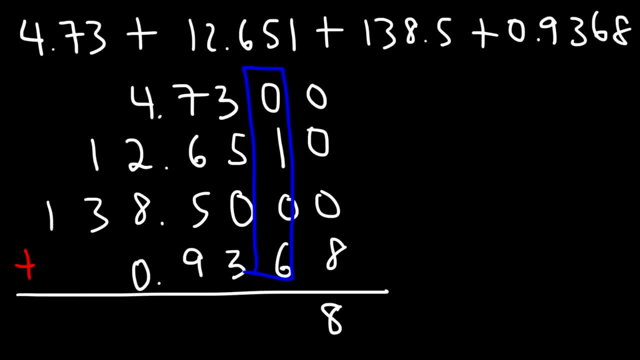 we can add a 6 and a 1, so that's going to give us 7. and then, for the third column, 3 plus 4 is 9.. 3 plus 4 is 9.. 3 plus 4 is 9.. 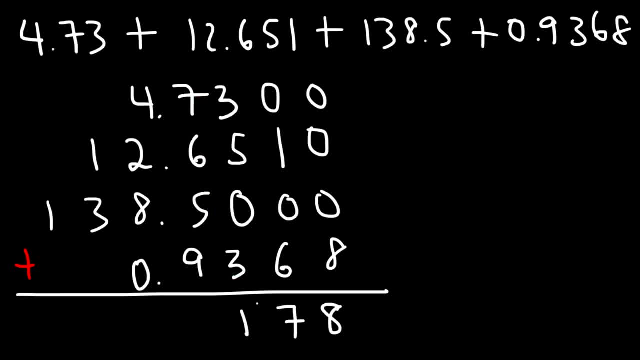 5 is 8.. 8 plus 3 is 11.. So let's write 1 and carry over the other one. So now let's add these numbers, So we have 1 plus 7, which is 8.. 8 plus 6 is 14..